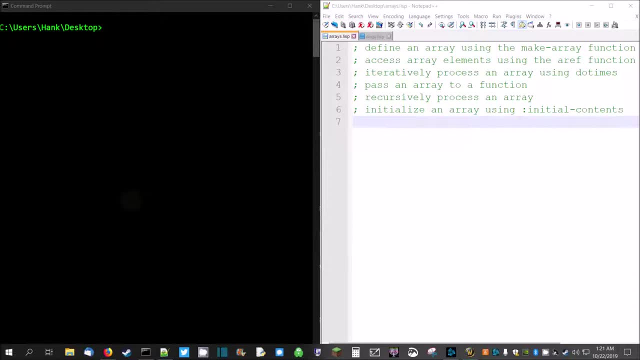 other programming languages. right, An array is an object that's going to have multiple elements. Each of those elements can be accessed using subscripts, and the subscripts are numbered as you're used to: First element's got zero. second element's got one. third element's got two. 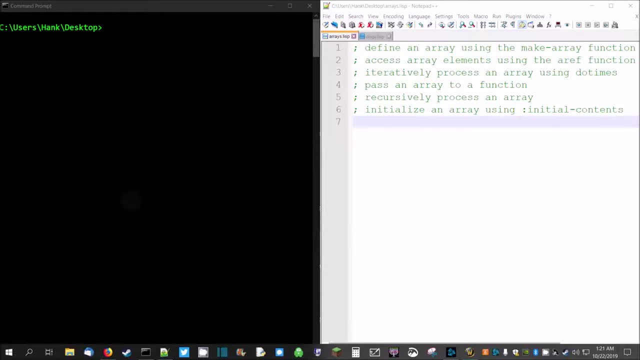 etc. Okay, so you know, these are array arrays. This is. you know, when you think about array, we're thinking about arrays. So this is, as opposed to lists, Arrays. depending on what you're using or what you're trying to do with, LISP may be easier to use than a list. 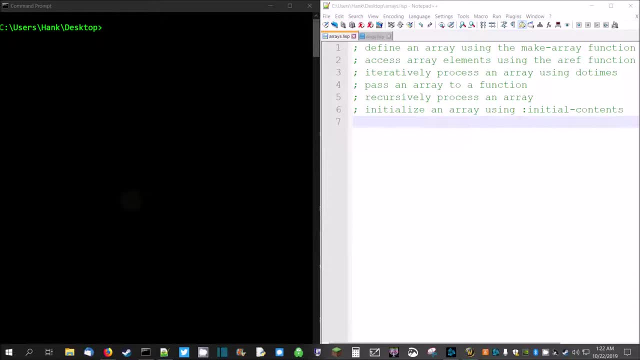 You know they both have their pros and cons, but the purpose of this video is to talk about how arrays work and give you some examples in LISP. Okay, so here's the things that I want to show you. I want to show you how to define an array, and to do that, we're going to have to use 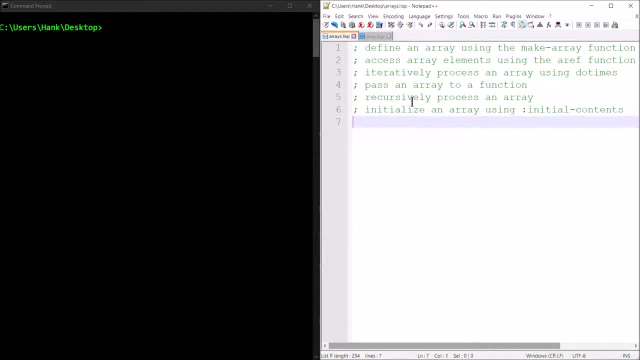 a LISP function called makeArray, and I'll show you how to do that. I want to show you how to access the array elements, and in order to do that, we're going to have to use the aref function. I want to show you how to iteratively process an array using doTimes. So doTimes is a 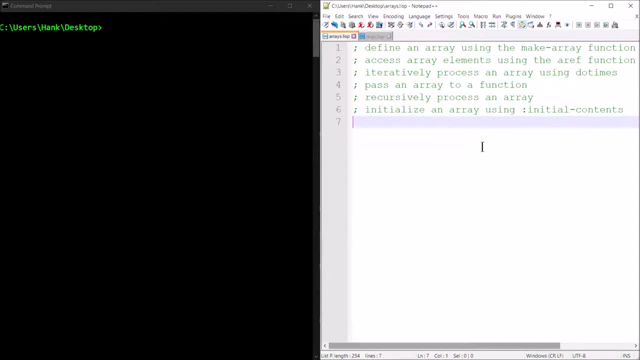 repetition structure or is a manifestation of a repetition structure in LISP. So I'm going to show you how to do that. So, basically, you know how can we step through the array one element at a time, starting at element zero, through, you know, n minus one. I'm going to show you how to pass an. 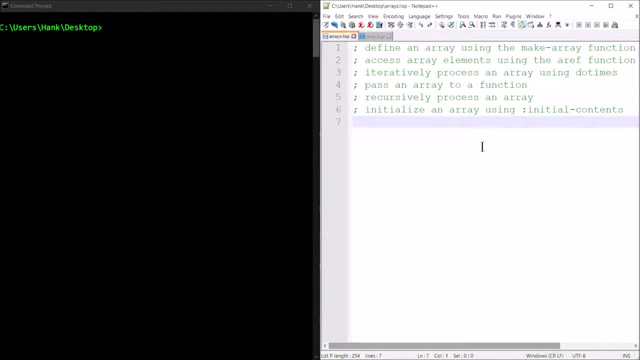 array to a function. You know it's surprise, surprise, spoiler alert. it's going to be just like you're passing anything else to a function. I want to show you how to recursively process an array. I want to show you. 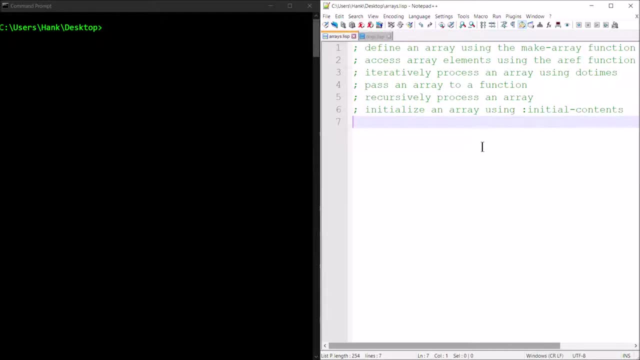 how to initialize an array using the initial contents modifier. So, if you remember, in languages like C++ you know they have that initialization list. Well, initial contents is similar, right? It serves kind of the same purpose in LISP. Okay, so let's go ahead and get started. 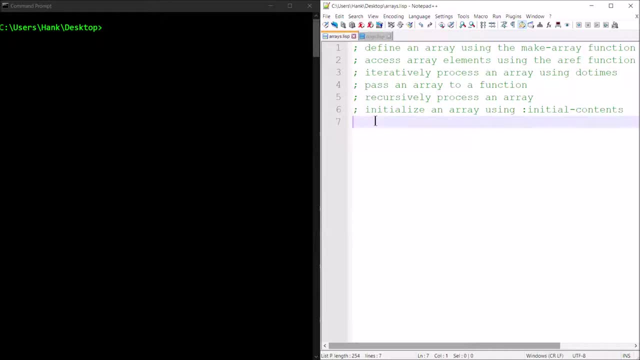 here. Okay, first things first. let's go ahead and define an array, right? So in order to define an array, we're going to have to use the make array function. okay, Now, the make array function is going to take as an argument a list, right? And so what goes inside of this list is going to be: 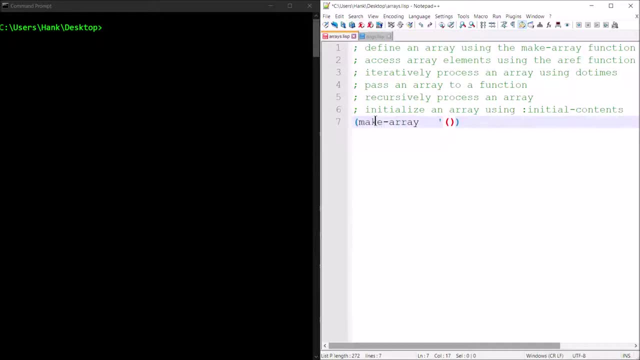 the number of dimensions that you're going to have, plus also how many elements per dimension. right? So, in this video, just going to do, just going to focus on one dimensional arrays, to keep it short, right? So if I wanted to create an array that contains five elements, right, I would just put. 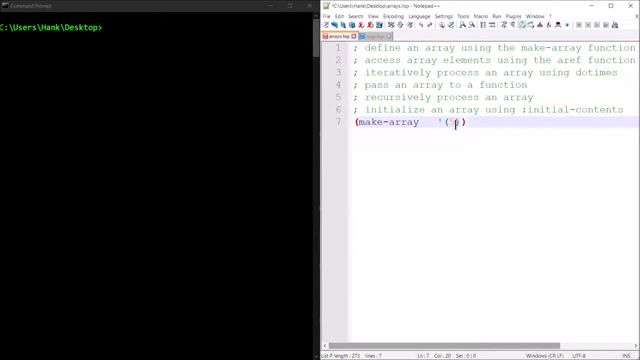 five inside of that list. Now, if I wanted to have a multiple element or, excuse me, a multi dimensional array, well then what I would do is I would add additional values in here, you know, for each dimension. So the first dimension would have five elements in it. the second dimension would have three. the third 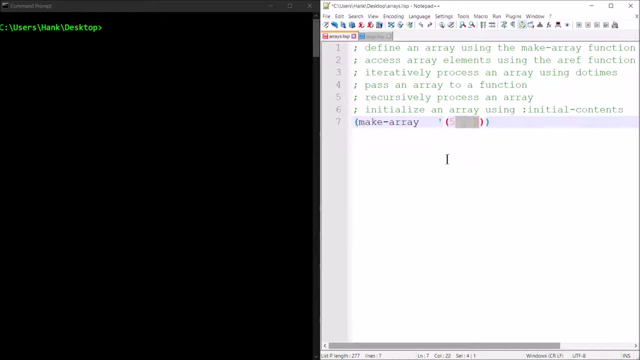 dimension would have eight, etc. right, But I'm only going to have a one dimensional array in this video, okay? So once I've done that, this is going to create an array of five elements. okay, Now, if I want to use that array, then I'm going to have to assign it to a variable. So I'll call this: 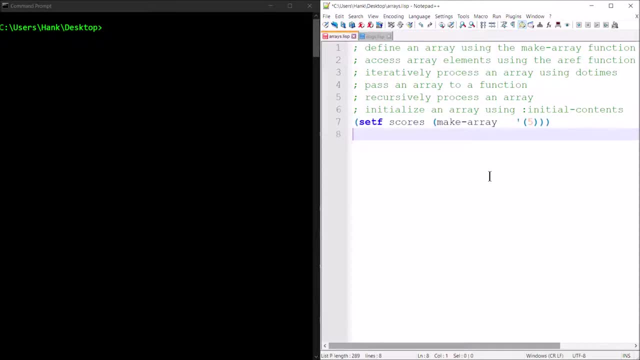 variable scores. okay, Now, if I was to go ahead and write the scores on the screen, right, this is what we're gonna have, right? So let's go ahead and run it. So you can see the output here: nil- nil- nil- nil. Hashtag means that this is the contents of an object and arrays by: 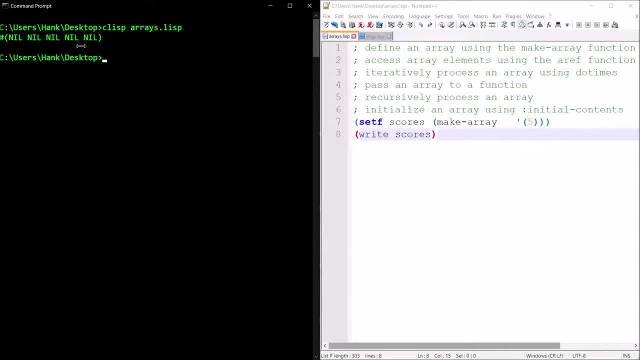 default get initialized with all nil, right, which is, you know, a Lisp version of either false or no. okay, so now what if I want to set some values in that array? right, if I want to access those array elements, put some values into those elements or get the? 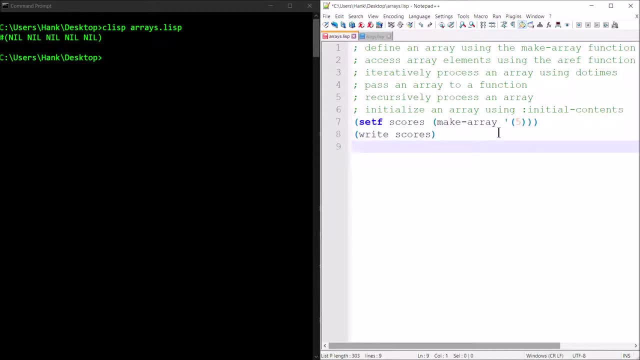 values out. okay, so what we do is we use set up and we use the a ref function. now, the a ref function takes as arguments the name of the array and the index that you want, or the index for the element that you want to access. right? so in this, 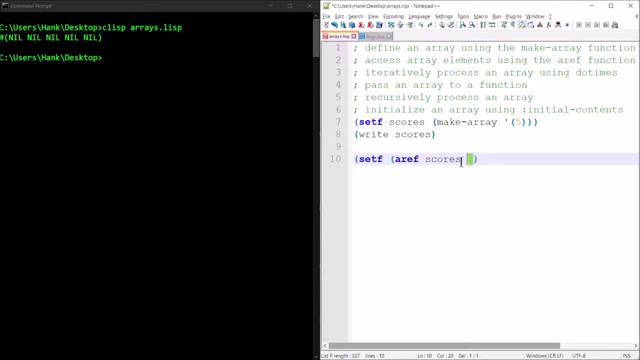 case. what I'm trying to do here is I'm trying to set the zer with element of the scores array to 87. okay, and likewise I'll set, you know, the other elements. so there's five total elements here. so element one I'll set to 95. element 2, I will set to 77. 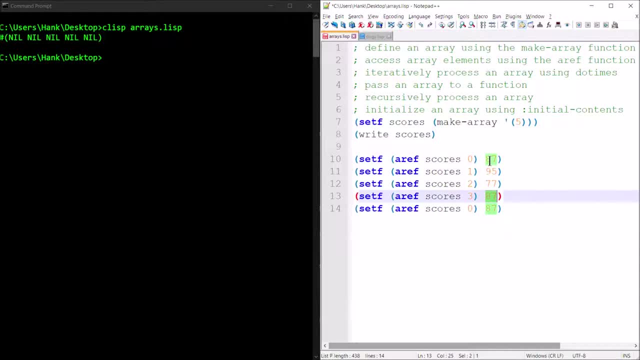 and on at three, I'll set to 84 and element four will set to sixty three. okay, so now, if I was to write out the contents of the array, right, we would see these updates right. so now, if I was to write out the contents of the array, right, we would see. 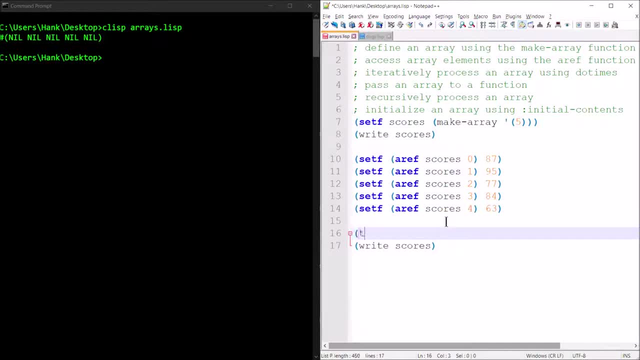 values. Now I want to have that output on separate lines, so I'll use the TERPRI command here, the TERPRI function, and that just moves the cursor to the next line. Okay, so let's go ahead and run this. All right, so this is before nil. 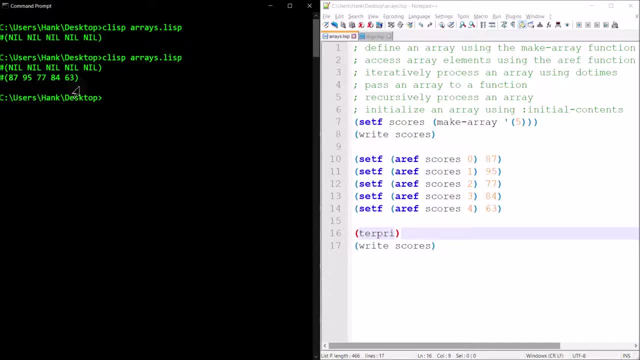 nil, nil, nils before, and then 87,, 95,, 77,, 84,, 63 is after. Right now. what if I wanted to access a individual score or an individual element? All right, well, let me move the cursor to the next line again, and then I could just do, you know, write. 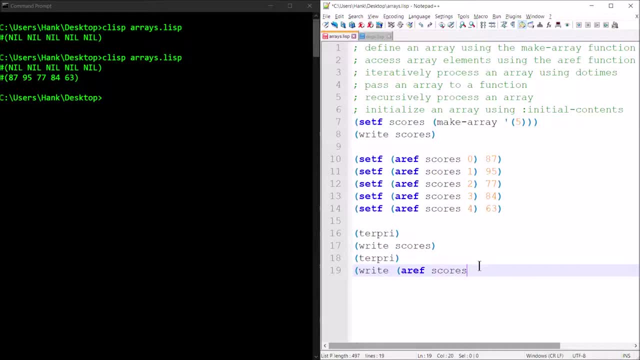 aref scores. Say I wanted to print 77 on the screen Right, just do something like this. So this is the aref function. It's saying: you know, in the array scores, give me that third element and then we'll pass it to write for printing on the. 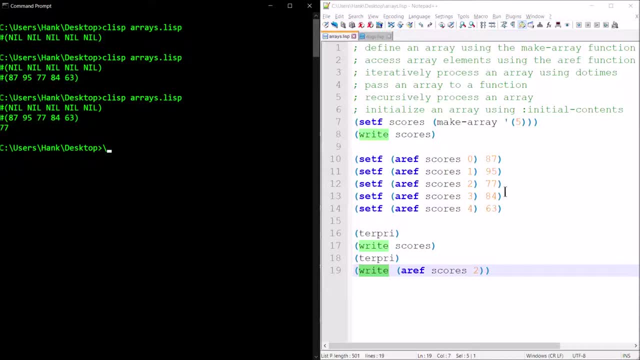 screen. Okay, so there's our 77.. Okay, now what if we wanted to process the array iteratively, In other words using a repetition structure, a loop? Well, we could use do times to make this happen. and let's say that I wanted to add up the total of all of the scores. 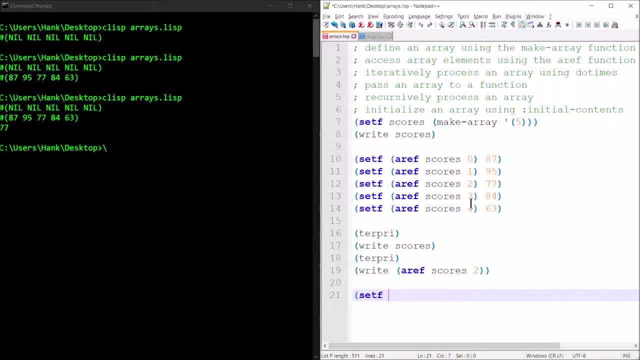 in that array. All right, so I'd want to create a variable called sum, right, and I'm going to initialize it to zero, okay, and then we'll print sum right, we'll run this, Okay, so let's go ahead. and you know, iterate, excuse me, iterate over. 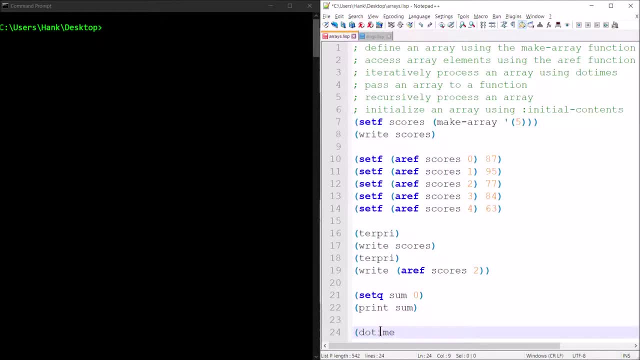 this array, So make that happen. I'm going to use do times right, and do times kind of looks like a function in that you know, you've got this word right here and you've got what looks like to be a parameter list here, but this isn't really a parameter list. this is what we're going to put. 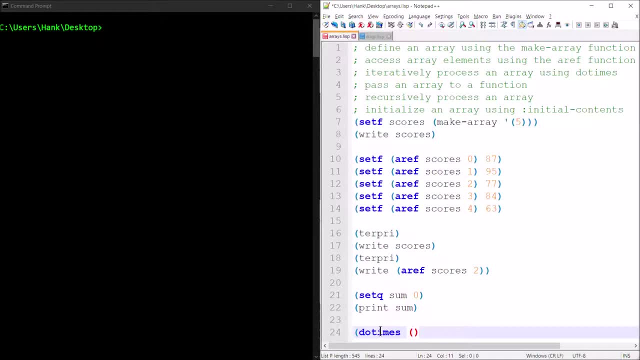 in here is we're going to put a variable and an integer, right. so you know, think about c++. you got four in. i equals zero, i less than five, right? well, there's the i and there's the five. 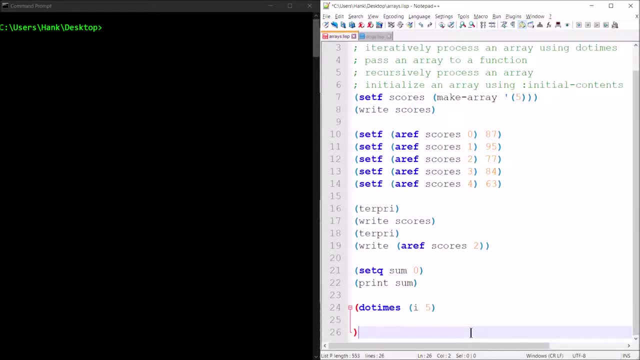 right. so why did I pick five? Well, because five elements right. so what I need to do for each repetition, for each iteration, is: I need to take what's inside of a ref scores of i right, and then I need to add that with sum right, and then, once I've added, 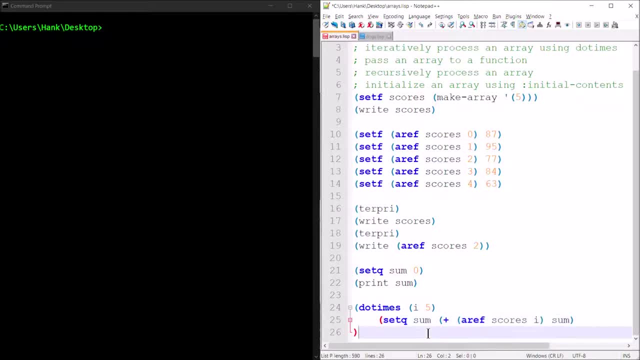 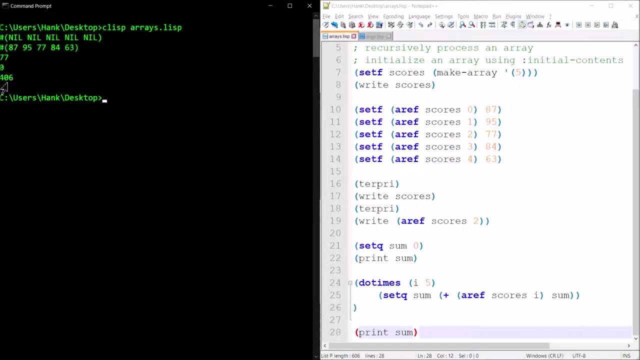 that with sum, then I need to update sum, right? so, just like that, Now let's go ahead and print out our sum To see the result, right? so let's go ahead and test this. right, so you can see. there's the total. 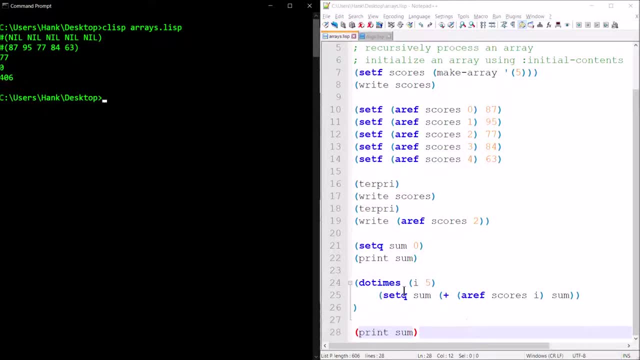 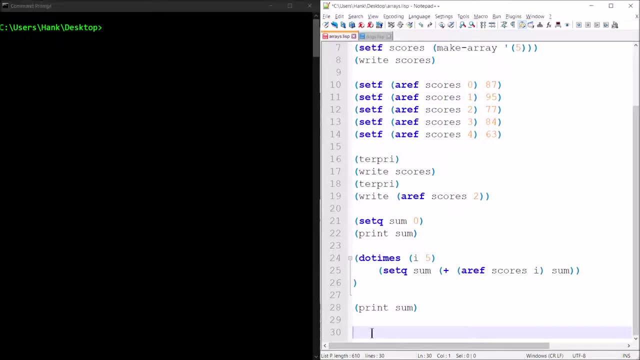 sum for the array, okay, okay. so what if I wanted to show you the average, right? so then what I would need to do is I would need to divide sum by five, right? and then maybe I'll assign that to a variable that I'll call abg. 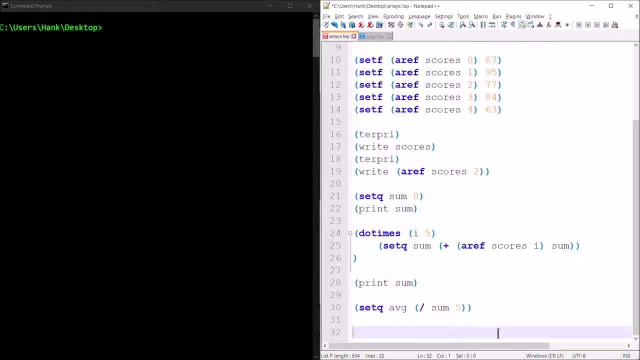 Okay, and then once I have that, I can print the average. okay, so let's run that and see what happens. so there's the answer: 406 fifths. right, I mean that's not wrong, but we probably wanted. 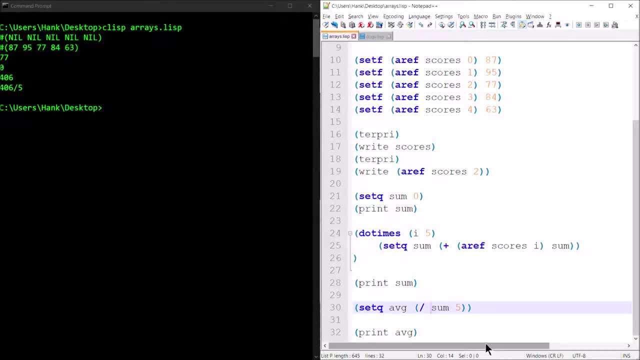 to see a floating point number, right. so if we're going to do that, then what we have to do is we have to convert that one of these guys. you know sum will do, or we could have done five, convert it to. 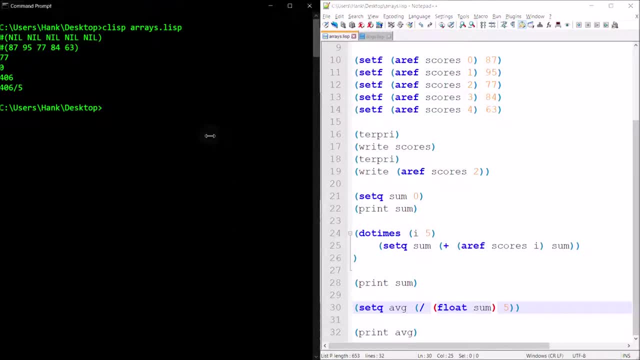 a floating point number, and so that way that'll force floating point division. right, and so now there's your average: 81.2.. All right, so how about passing an array to a function and you know doing something with the. 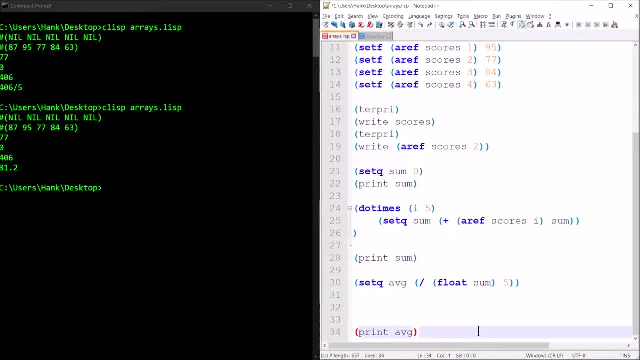 array inside the function. well, let's go ahead and do that. so right now I've got scores, you know all these values in it. right here, I wanted a function that would set all of the elements to say 99, right. so what could I do? 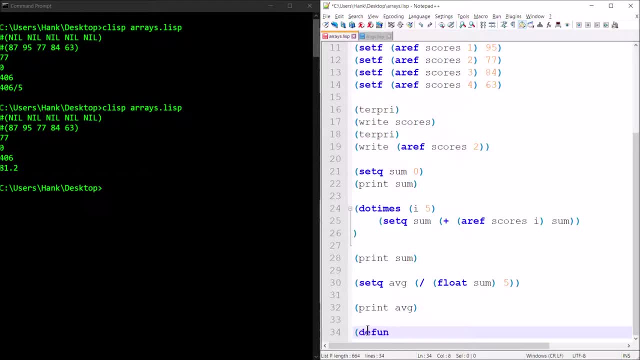 okay, so what I could do is I could create my function and I can call this whatever I want, set elements to 99,, I guess, and my parameter list. I'll have a parameter for the array and then also a parameter for the length. 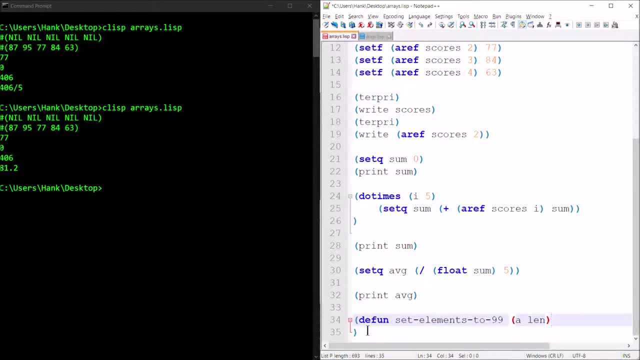 of the array right. so for this function I'll make it an iterative function. it won't be recursive. we'll do a recursive function here in a second, but I could use that do times again right. and inside of here I'll have i for my, you know, my counter variable, like I had before. 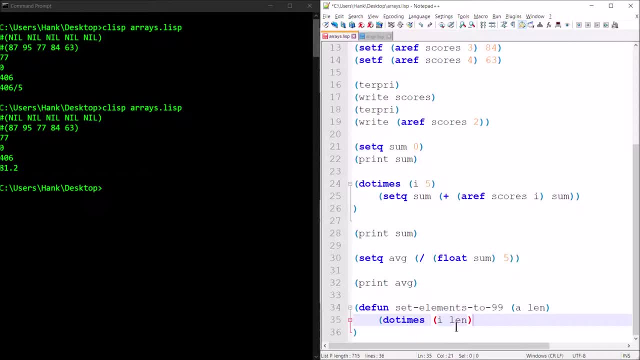 and then I'll use len here for the number of repetitions. I'm going to have half right. so once I've done that, then it's just a matter of updating each one of the elements of the array right? so set f aref scores of i- well, not scores, excuse me- a right, because 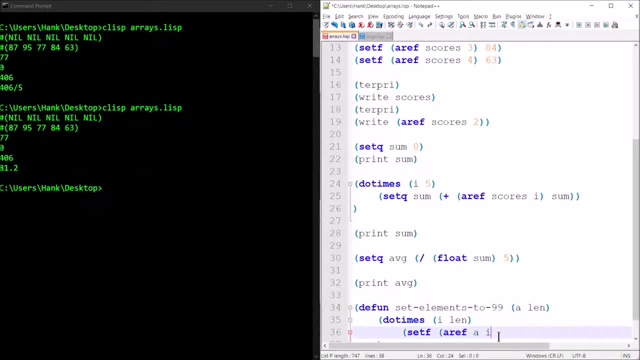 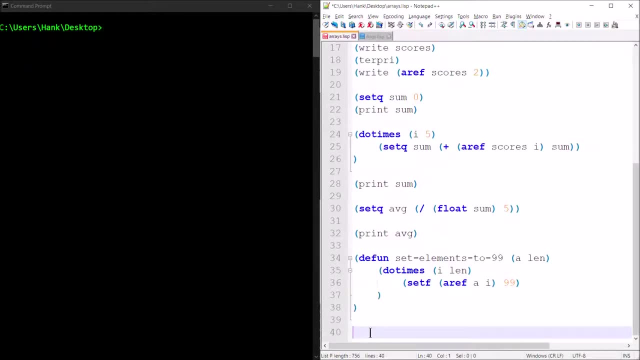 we're passing it as an argument, okay. so what do I want? to set that to 99,? okay, and that should do it. okay. so now that I have that function defined, I'll go ahead and call it right, set elements to 99, and I'll pass to it as an argument or as arguments. 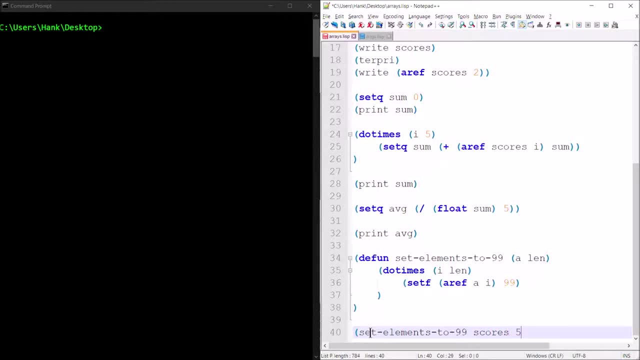 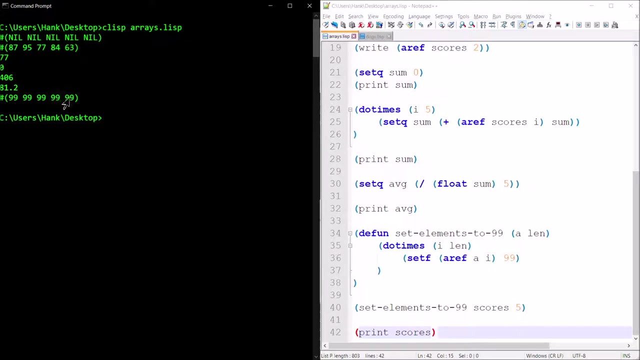 the scores array and the length of the array, which is five. okay, and then I'll print scores, okay, and then we'll go ahead and call it, and so now you can see that the scores array is all 99s. 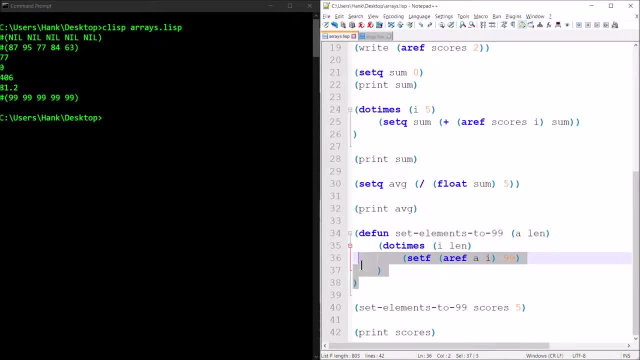 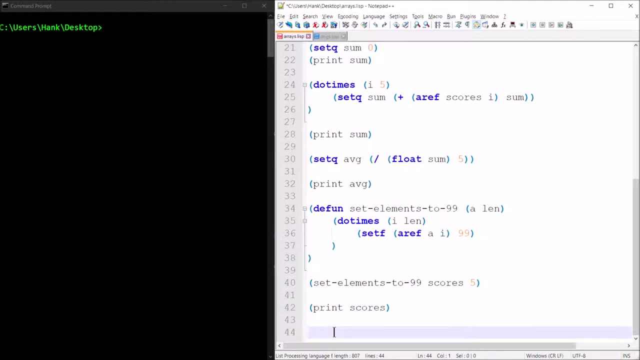 so, basically, what you have here is an example of the way this is behaving- is passed by reference, essentially, right, okay, all right. so let's see an example of a recursive function that processes an array, right, so what I'll do is I'll recursively add up the sum. 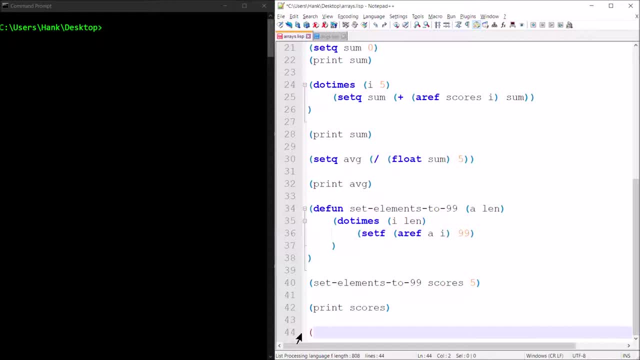 of the array that'll pass. it'll pass the scores array, so that's the one we have right now. line that up using recursion and what we'll do is we'll- well, let me go and get started. okay, so we'll define. you know, call this recursive sum right in our parameter list. 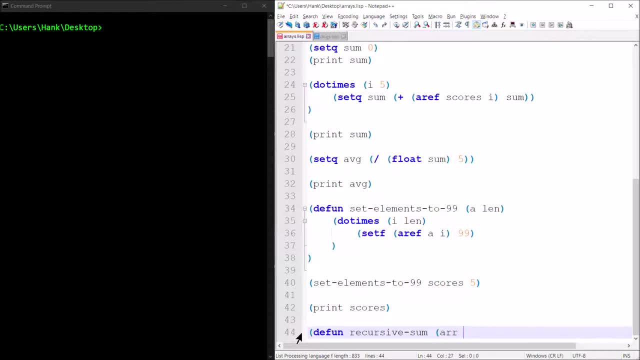 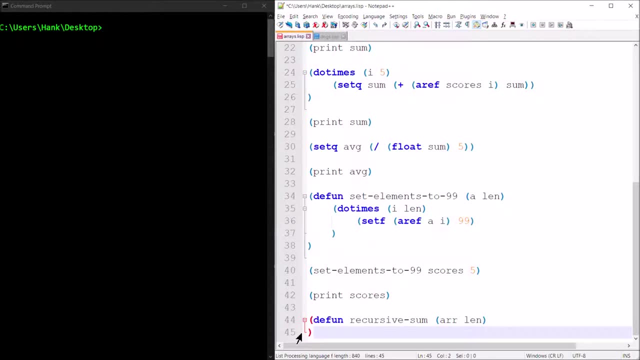 we're going to need one parameter for the array. we'll call that r, and then we'll need another parameter- I'll call it len- for the length of the array, right? so when we call this function, we're going to pass it the array and how many elements that it has in it. 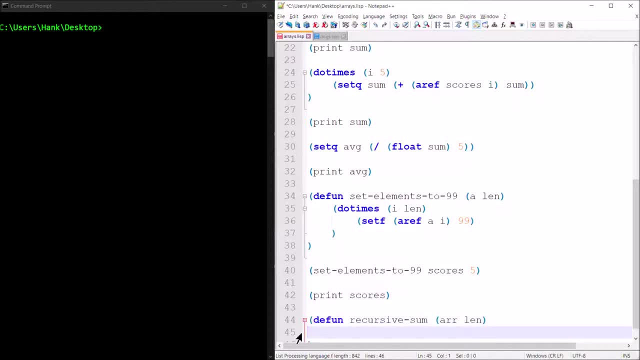 so what I'm going to do with this is I'm going to add the array up kind of backwards right, because plus doesn't matter. so you know, if I add up element first, if I add up elements four and three, right, it doesn't matter if I do that or if I add up elements three and four. 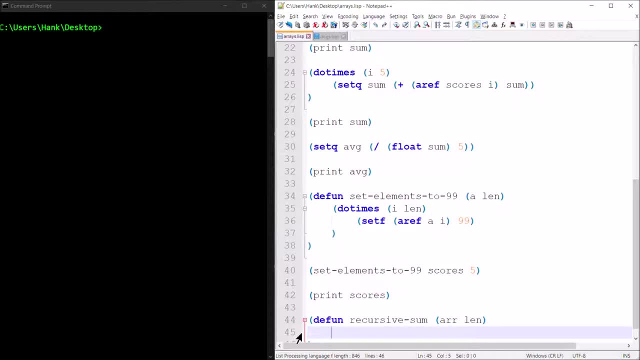 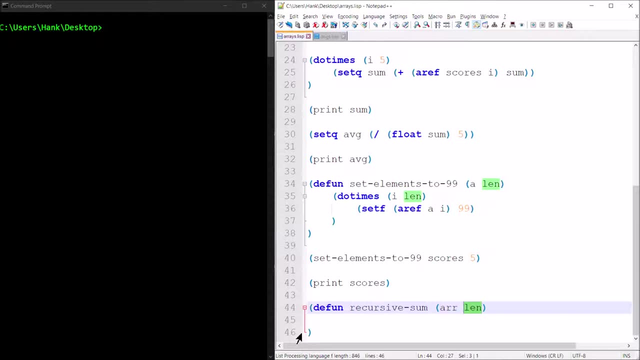 that order doesn't matter, right, and so by doing this I can save myself a variable. so I'm going to use len. initially it's going to contain the length of the array, but then it's going to become essentially a counter that's going to control how many. 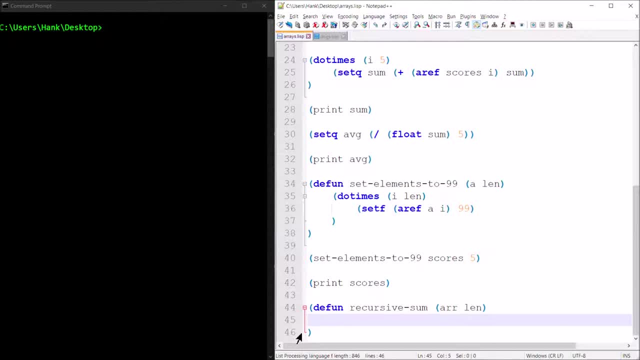 repetitions we have okay anyway. so initially I pass five as an argument. well, five's not a valid index. so what am I going to do? I'm going to call the def function and what that does is that allows you to specify a variable that you want to subtract something from. 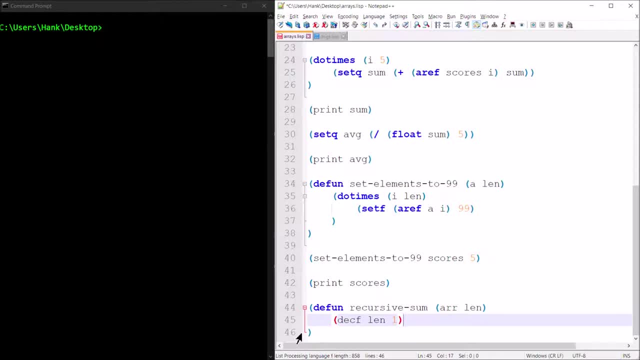 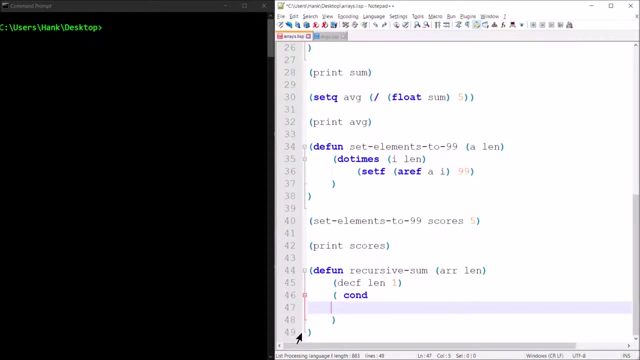 and I want to subtract one right, because pass five initially, subtract one from now. len's got four in it. that's a valid subscript. I can work with that, okay. so then I'm going to need my decision structure in here. I'm going to use con right because, remember, con is like a. 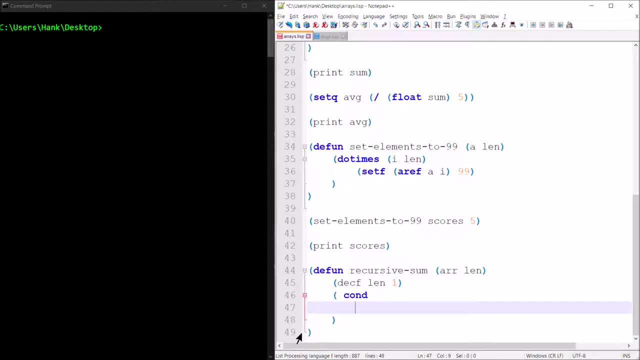 if else, if type structure. and what I want here is I want to have a base case. so if len is less than zero, right, then I'm out of here, right. there's nothing more for me to do, so I'm just. 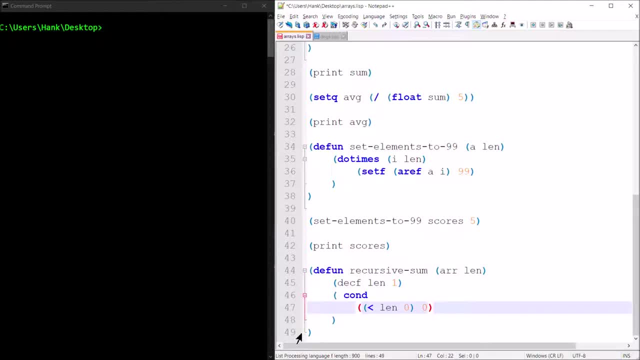 going to return zero, Right. so if len is less than zero, I'm out right. because if len is serving also as my subscript for doing my traversal of the array, negative one or any negative number is going to be an invalid subscript, right? so I'll just return zero and then the function will be over. 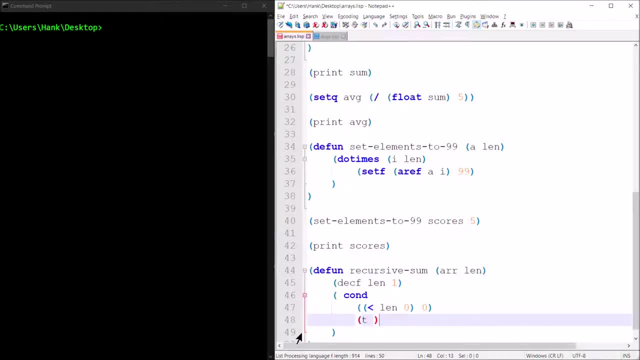 that'll be my base case, okay, otherwise I'm going to need to do something else. and what's that something else? well, I'm going to have to add the element at index len to the sum of the rest of the array, right? so I'll do this. I'll say aref. 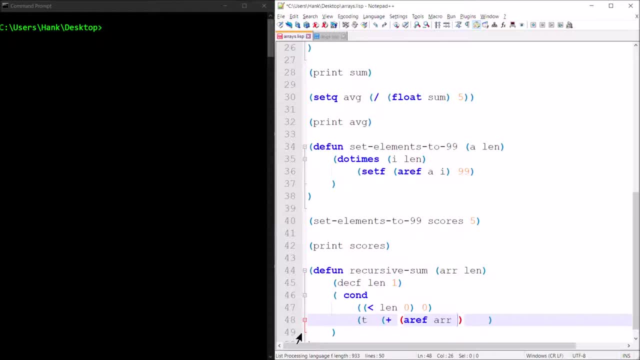 r and I'll use len for my index, right? so len's going to be four, then three, then two, then one, then zero, no problem, so I'll be able to extract each the contents of each element. 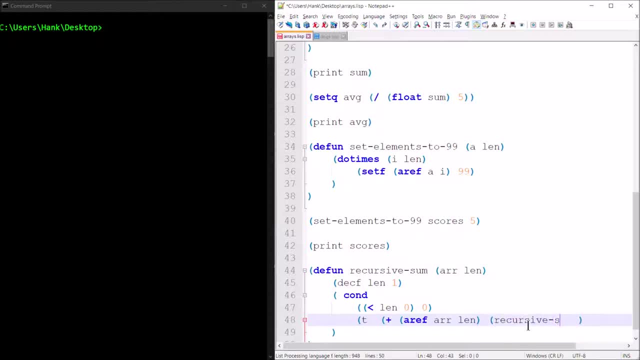 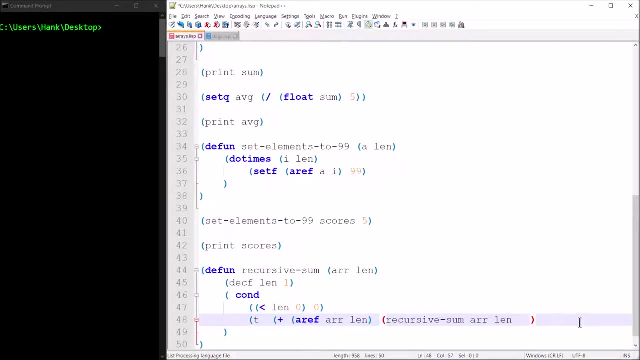 and then I can add that to- and here's my recursive call the rest of the array. okay, so that should do it. let's make sure that our parentheses all match here. I might be missing one. I think I am actually right, so I need one more there. 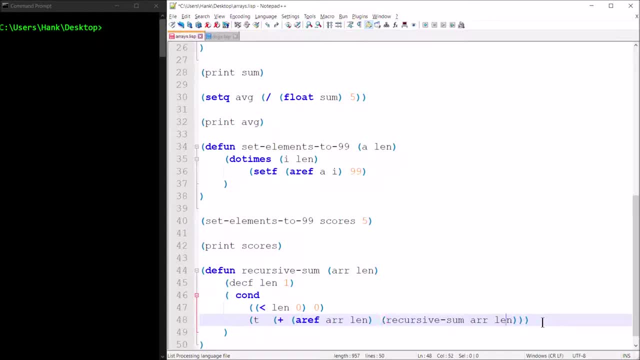 and one more there, right? so let's see here. so what am I doing if this is false? we kick down to here and then we do our addition, right right there. and what are we adding? the contents of the length element of the array and the sum of the rest of. 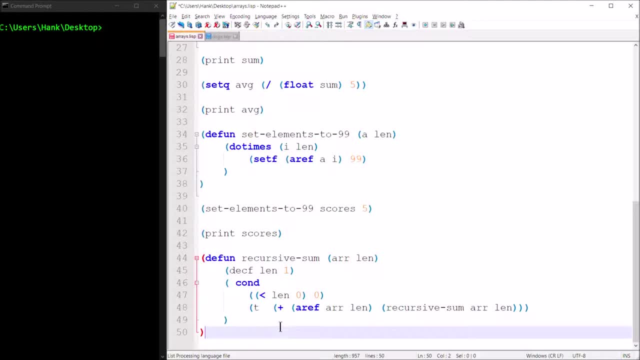 the array right. so I think that that's everything that we need there. so let's call the recursive sum, we'll pass it scores and we'll pass it five, because there's five elements right, and then I will put what's returned by that function into a variable. 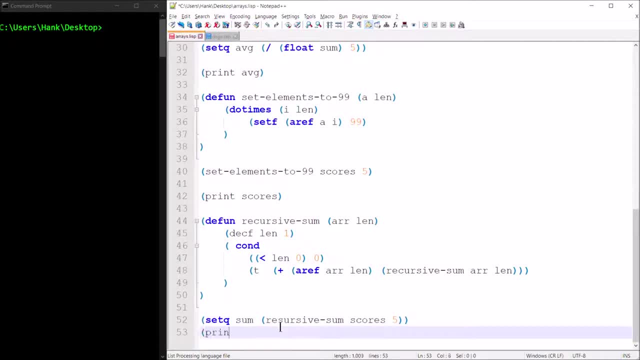 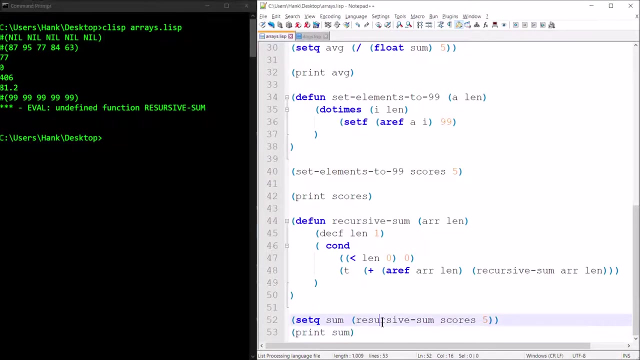 right into sum and then I'll print out the sum for you, okay, so let's give that a shot. see what happens. see what we got. all right, oops, made a typo: recursive sum. okay, let's try. 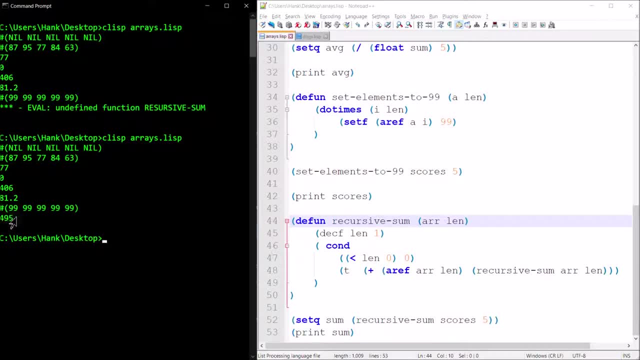 that again all right. so there we go. so there's our answer: 495, right. 99 times five is 495, so five 100s would be 500, there's a minus one for each one of those hundreds. 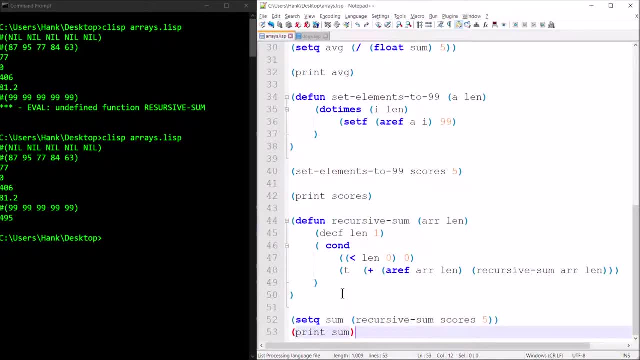 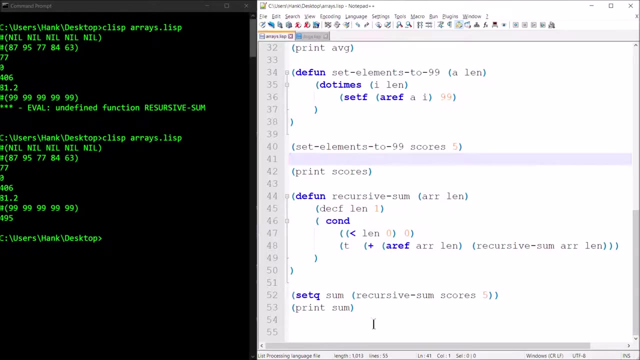 subtract five: 495,. okay, so there's a recursive function that adds up the sum of an array. okay, now one last thing here, and that is: how can we initialize an array? okay, so the way we're going to initialize an array is by using this modifier. 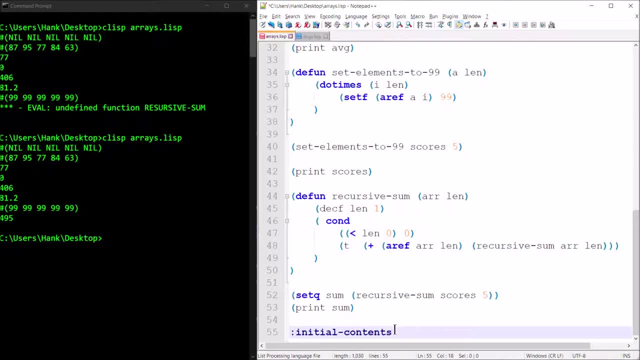 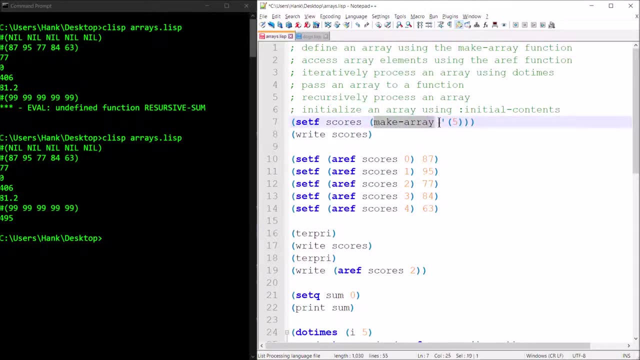 initialize no contents. okay, we're going to use this guy right here and we're going to include that with our make array function, right, so let's go ahead and just I'll just reuse this right here. right, so grab this guy and I'll use a different array name. right, so we'll call it. 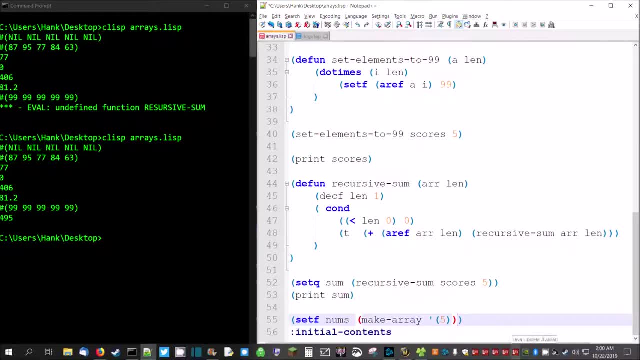 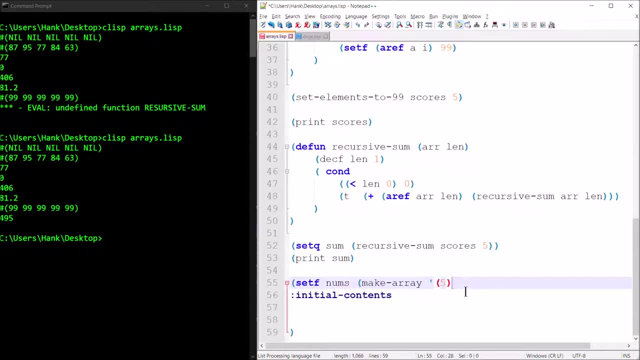 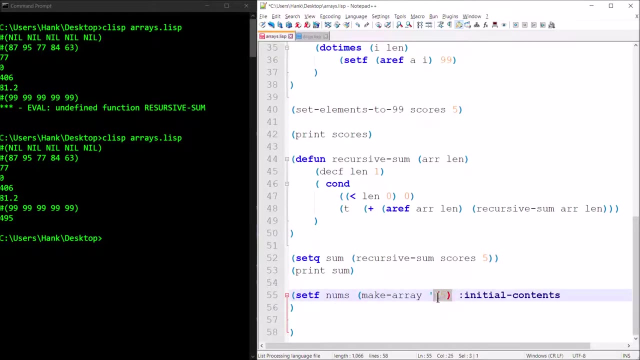 nums. fine, okay, and so what's going to happen is is is that we are going to set initial contents right and that's going to go after the- I guess you can call this thing the size decorator, right? I mean, this is going to be how many elements you're going to have in it, so 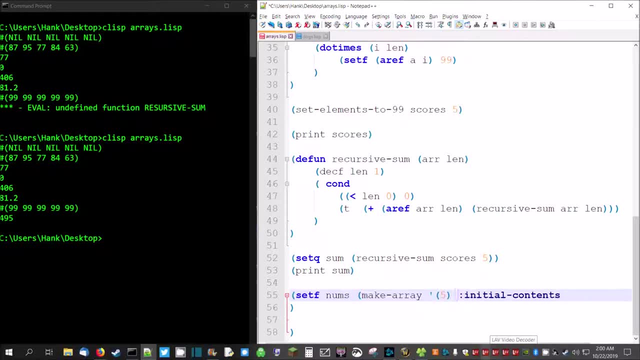 we put initial contents right after that and see, you'll see in some, you know, if you, if you google, you know this for extra supplemental information. whatever, you'll see that a lot of times people in sample code like to put initial these, these modifiers on the next line. 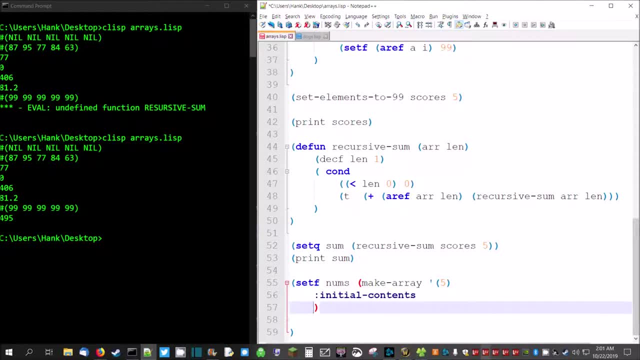 makes it easier to read. okay, fine, you know, not a problem with that. so what's going to come after initial contents is going to be a list of the values that you want in each element, right? so I've got five elements, and so I'm going to have five items in this list, okay? so once I've done that, 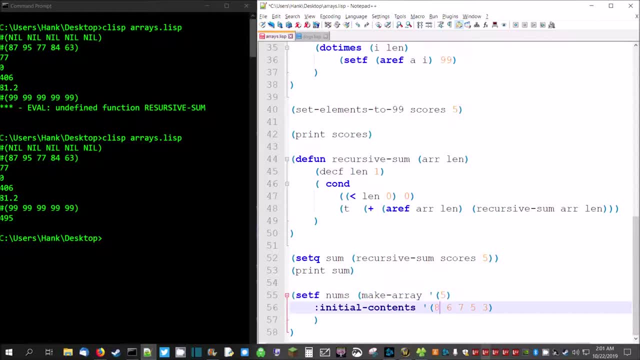 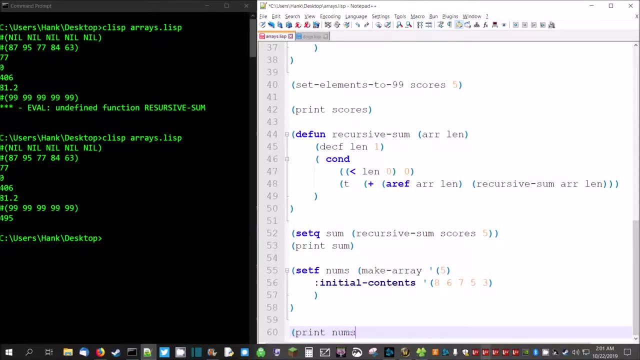 then I've got an array- five elements, and the contents are 8,, 6,, 7,, 5,, 3, right, and so let me go ahead and print out nums for you, just so you can see what this thing looks like. 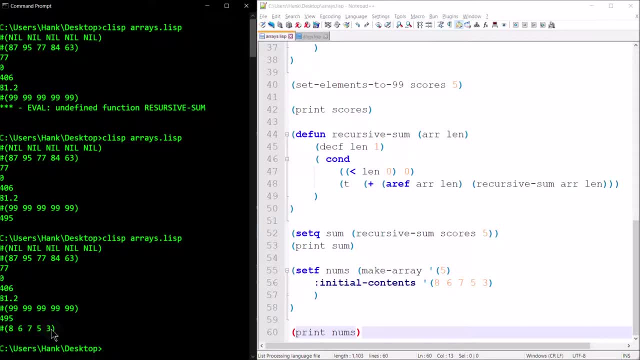 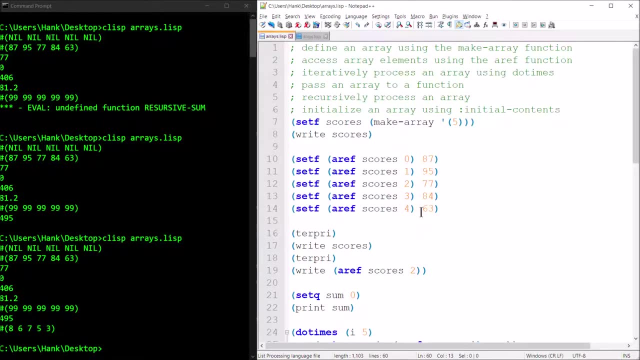 okay, so you can see. you know there's the contents of the array 8, 6, 7, 5, 3, okay, so I think that that's everything that I wanted to cover in the video. 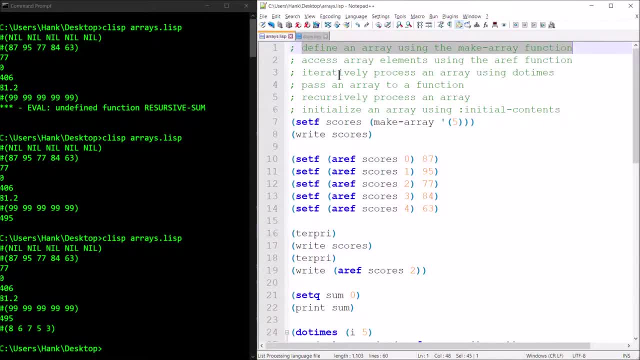 So I showed you a lot of stuff: how to define an array using the makeArray function. showed you how to access array elements using a ref. I showed you how to iteratively process an array using doTimes, using a doTimes loop. 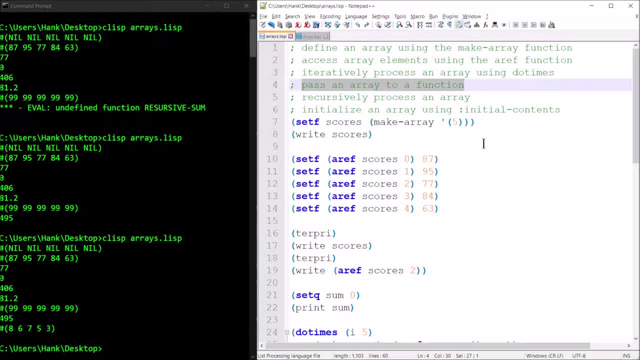 showed you how to pass an array to a function and demonstrated that they're passed by reference. Okay, I also showed you a recursive function for adding up the contents of the array, and I showed you how to initialize an array using the initial contents modifier. 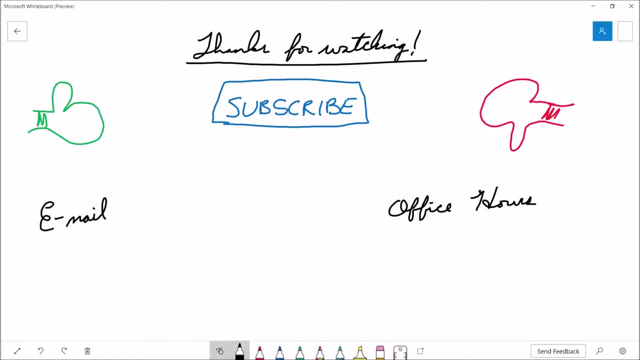 Okay, so that's going to bring this video to a close. If you felt that the video was useful, please consider giving the video a thumbs up, and if you thought that the video sucked, well then you've got that thumbs down button as an option as well. 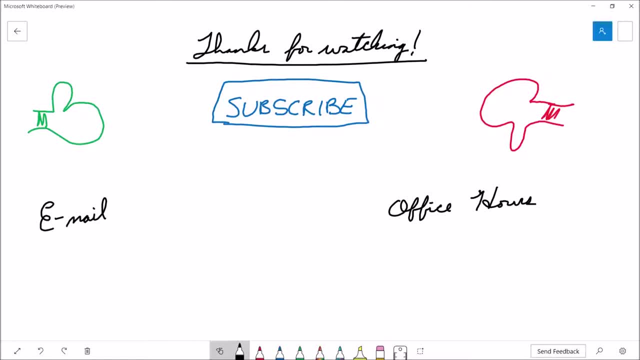 If you'd like to see more videos, if you're interested in more content from the channel, feel free to hit that subscribe button and, as usual, if you're a student of mine and you have further questions, feel free to drop me an email or to stop by my office hours. Okay, thanks for watching and we'll see you next time.